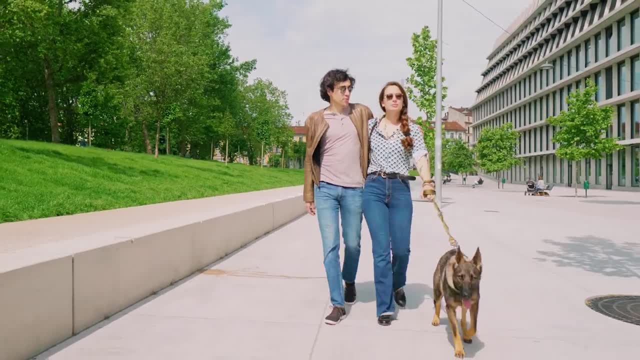 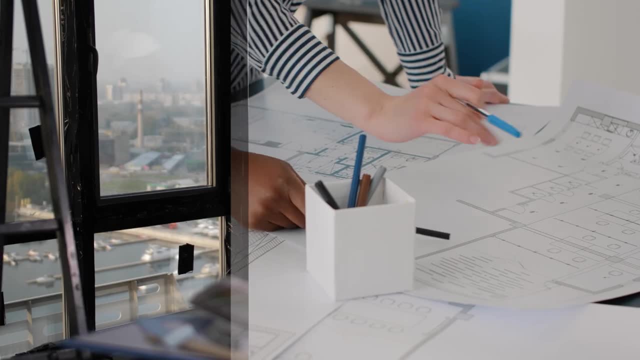 not only responsible for the environment, but also have a high standard of living, without compromising the ability of future generations to experience the same benefits. In order to achieve these goals, cities can utilize sustainable design initiatives, such as by using zoning policies to incorporate mixed land use developments into urban areas. 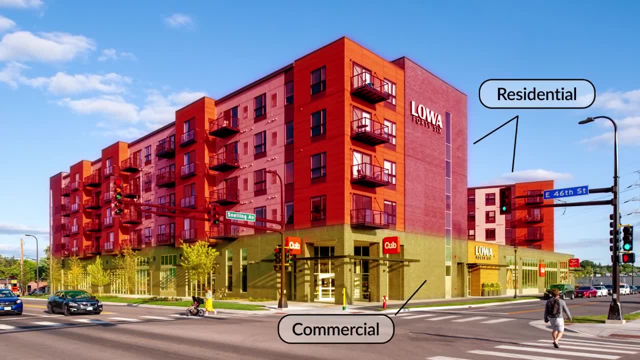 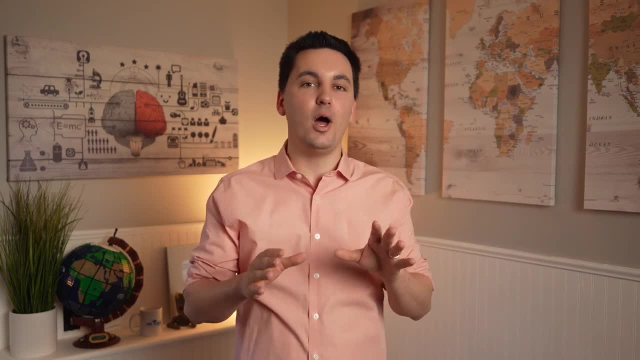 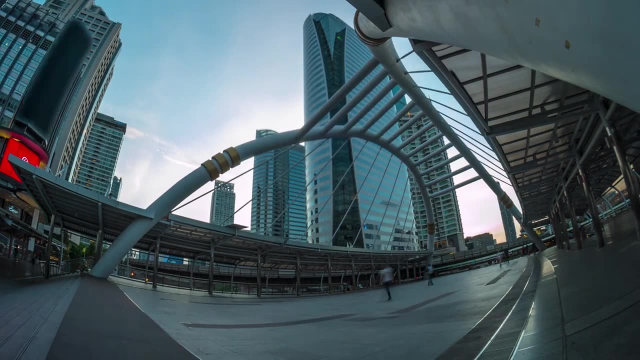 Mixed land use areas allow for the mixing of commercial, residential and sometimes industrial zones. This helps create neighborhoods where residents can work, live and play all in one area instead of having to commute between different places. This helps promote walkable cities, which are cities that design their city in a manner to decrease. 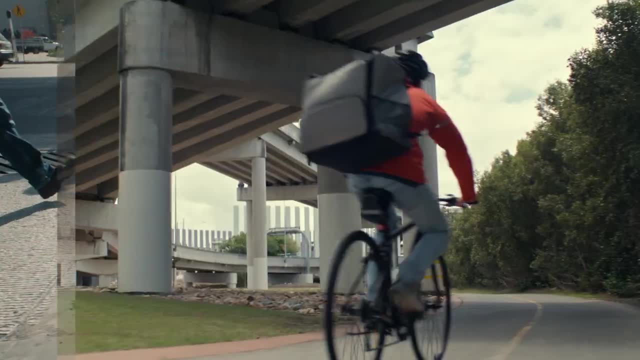 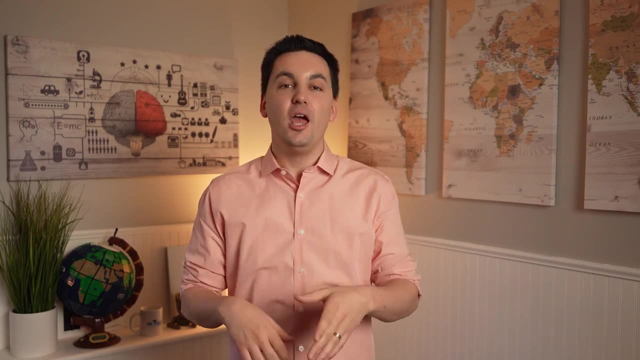 driving time and increase the amount of individuals who walk or bike to their destination. One of the ways in which cities can make it easier for residents to get from location A to B on foot is by utilizing smart growth policies which seek to promote compact 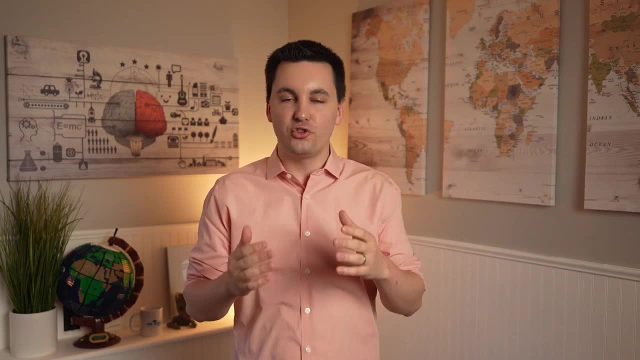 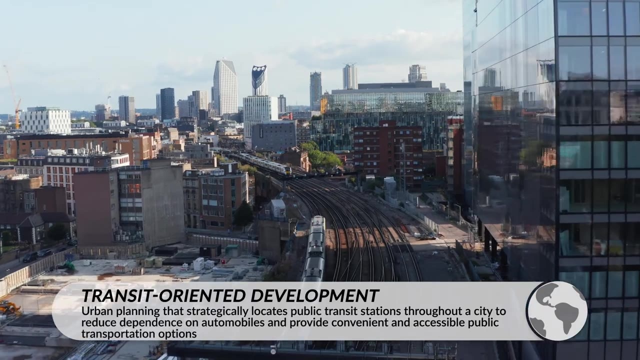 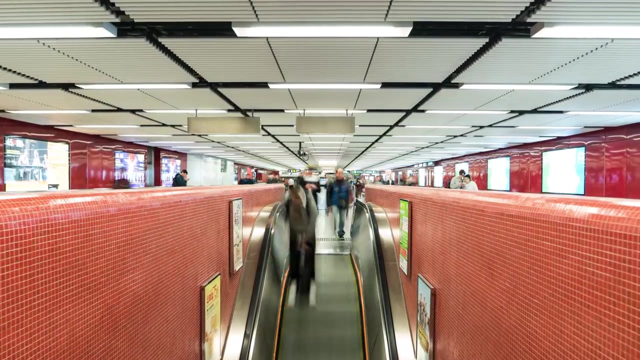 walkable cities, mixed-use building developments and zoning changes to reduce urban sprawl. Sustainable cities often prioritize transit-oriented development, A planning approach that aims to encourage the development of mixed-use areas and public transportation. This is done by strategically locating public transit. 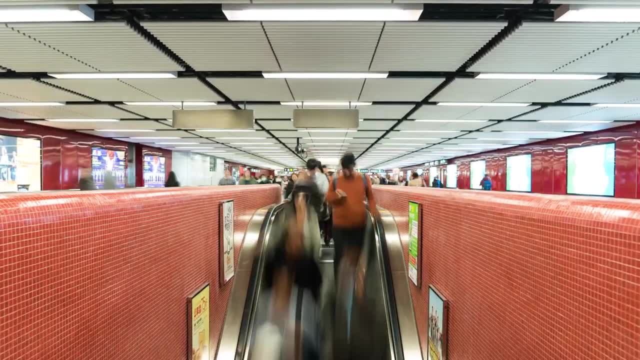 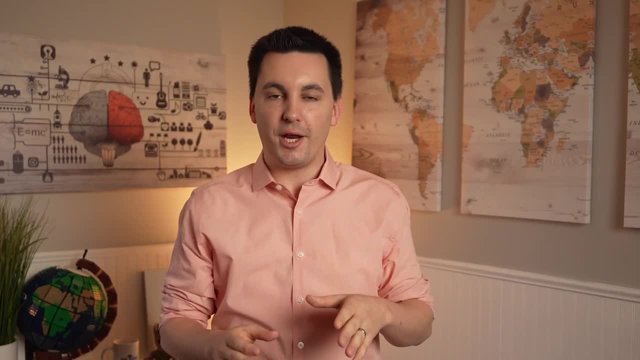 stations throughout a city, often resulting in a decrease in traffic and an increase in the use of public transportation. Plus, it has the added benefit of making the city more walkable. Now, before we continue on, I do want to highlight the difference between smart growth policies and. 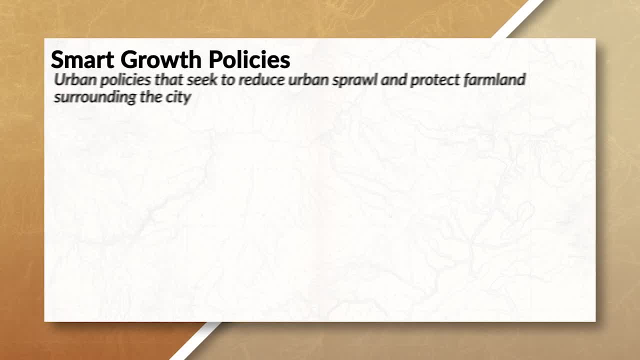 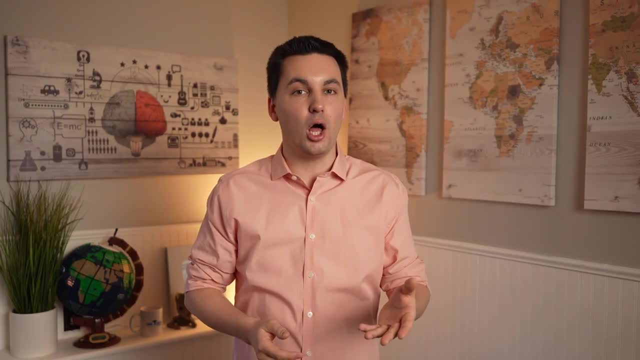 a concept known as new urbanism. Smart growth policies are policies that are focused around keeping an urban area compacted and safe for residents to use in their city. Essentially, the goal is to put the brakes on urban sprawl and stop the urban area from expanding. 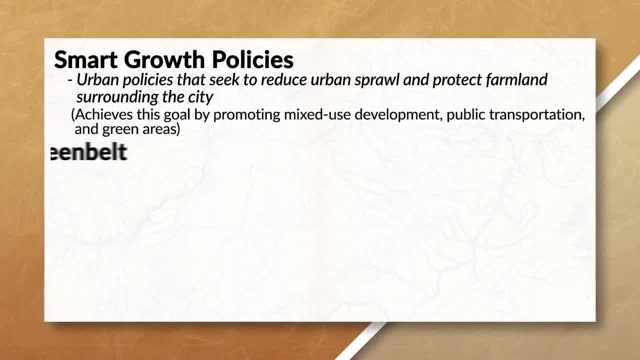 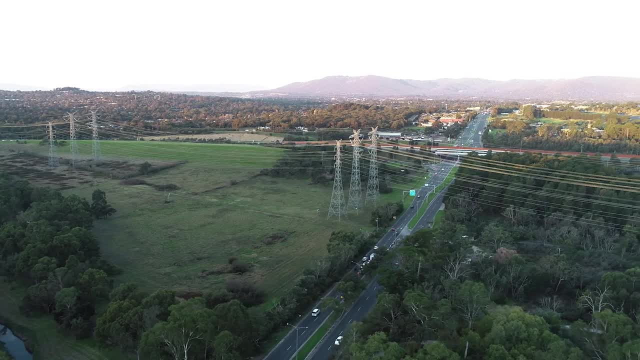 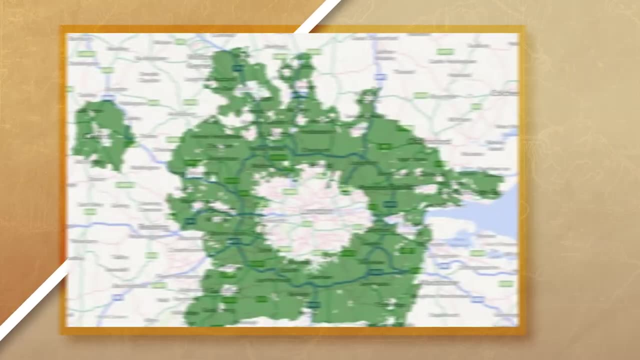 into the surrounding countryside. Smart growth policies can lead to the creation of greenbelts, which are undeveloped areas of land surrounding an urban area. These are intentionally left underdeveloped in order to preserve the environment, limit urban sprawl and provide a buffer between the urban and rural areas. When looking at greenbelts today, 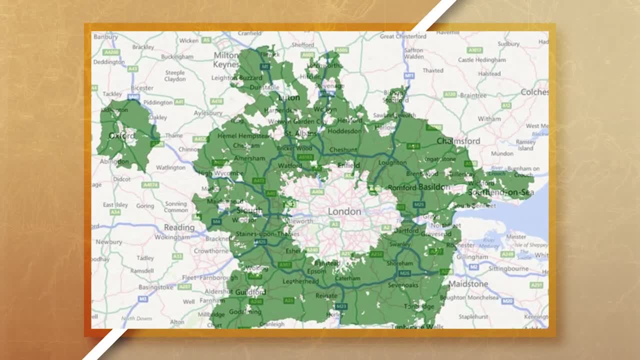 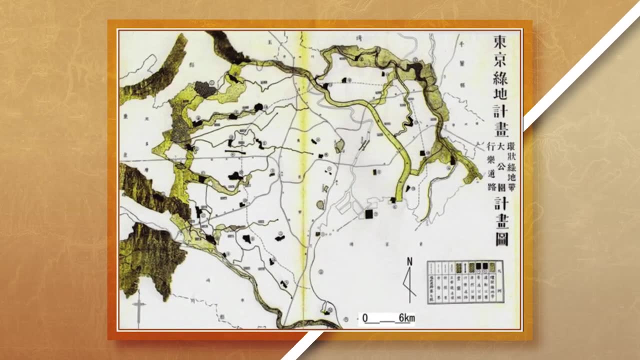 we can look at the London Greenbelt, which is estimated to have over a million acres of land, The Tokyo Metropolitan Greenbelt, which protects green spaces and agricultural lands that surround the city of Tokyo. Those are just two quick examples of greenbelts. There's more examples. 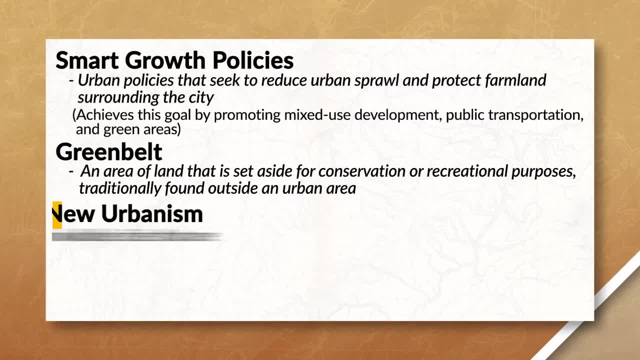 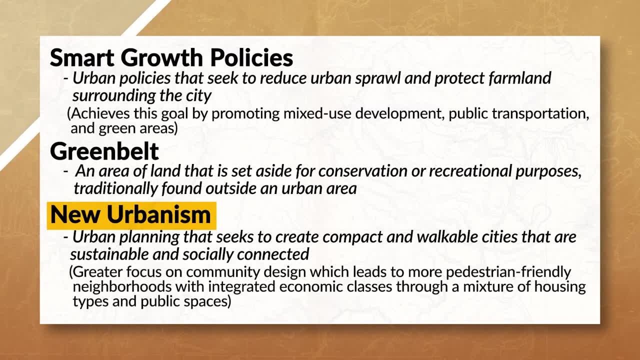 that you can find in almost every country around the world Now. new urbanism, on the other hand, also strives to have a more compact and walkable city. However, there is a greater focus on the architecture and community design. New urbanism puts a greater emphasis on community design. 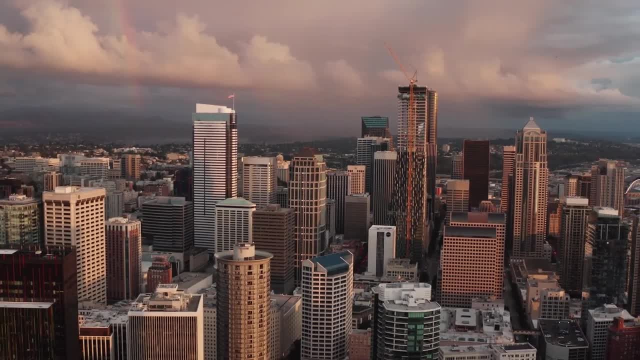 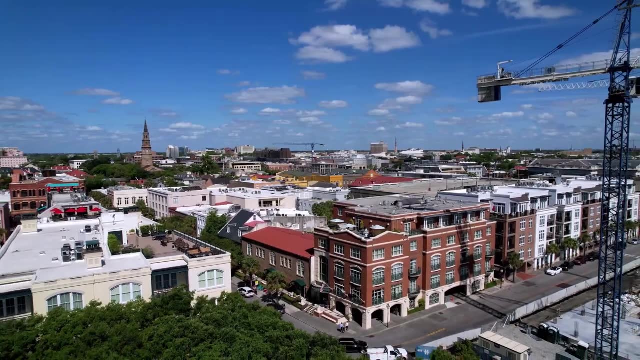 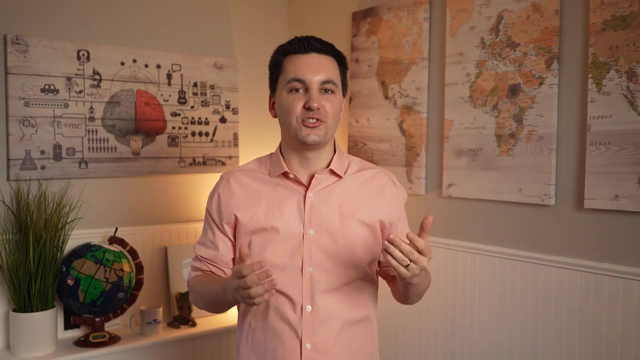 which often leads to more self-contained and pedestrian-friendly neighborhoods, which integrate economic classes through a mixture of housing types and costs. New urbanism often reflects European urban life, which puts a focus on local communities. Today, there are a variety of criticisms for urban design initiatives such as smart growth policies, As 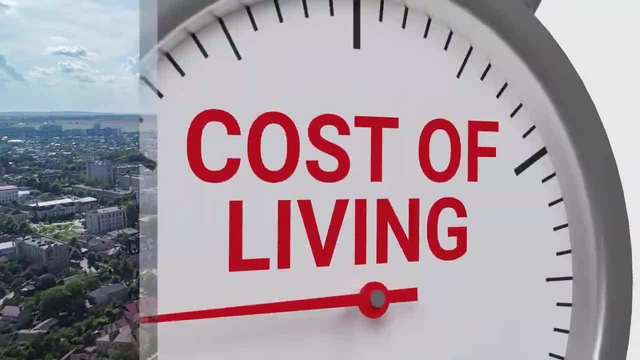 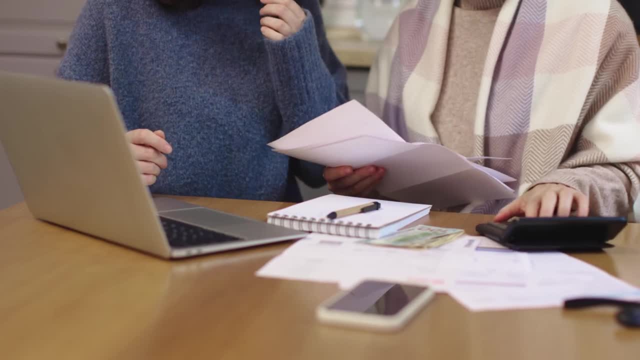 cities experience improvements in the livability and a reduction in the sprawl, it can cause the cost of housing to increase, which can end up pricing lower-income residents out of their homes and the city, resulting in de facto segregation. Segregation refers to the separation of people along racial 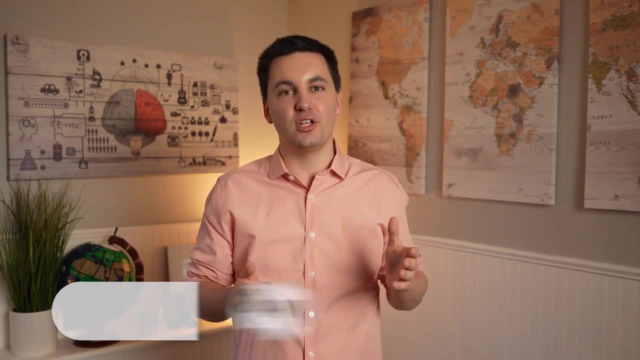 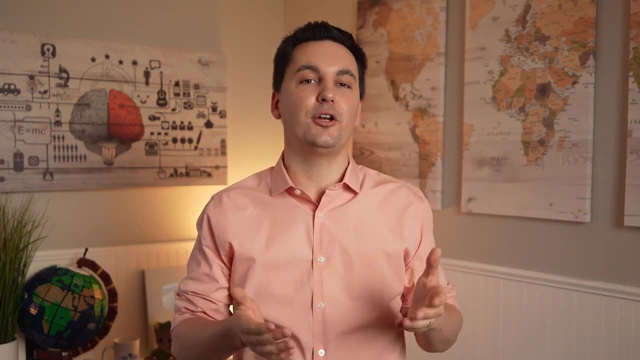 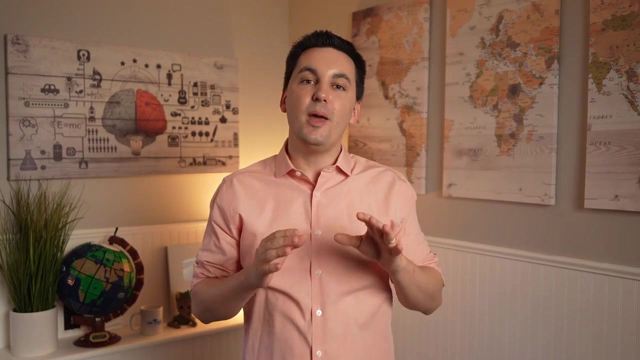 ethnic or socioeconomic lines that is not officially enforced by laws or regulations. Essentially, it's segregation that happens not because there is a legal law enforcing it, but because of unintended consequences. For example, as urban areas continue to improve and cities invest more in local infrastructure, it may cause rent and home prices to increase. resulting in residents who originally lived in the area to no longer be able to afford their higher mortgages, property taxes or housing prices. This may also lead to a decrease in taxes and other increases in costs, all of which increases the likelihood that the lower-income residents will have to move out of the area Plus. at the same time, we can also see that oftentimes, as urban renewal occurs in a city, we'll start to see more affluent residents move into the urban neighborhood, which may further displace lower-income residents. 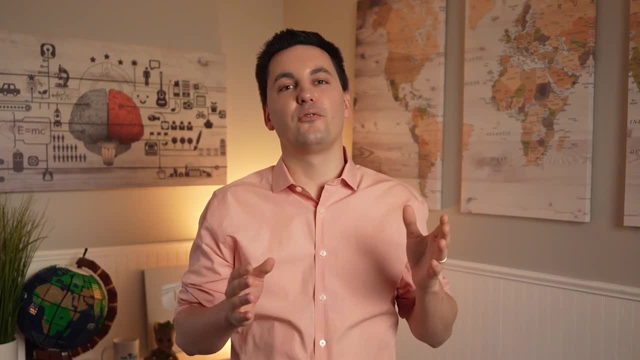 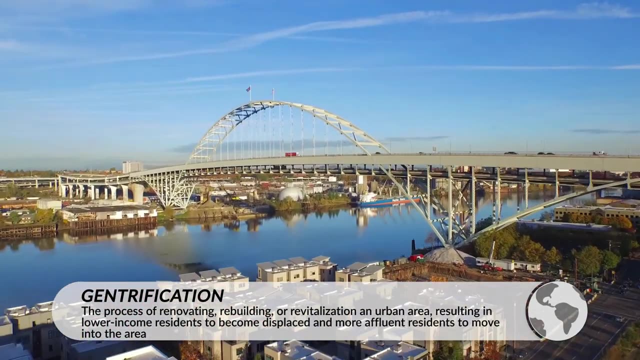 who have original community ties in the area. This is often referred to as gentrification. We can see an example of gentrification and de facto segregation in Portland, which is where we see a significant decline in the number of residents living in the area. 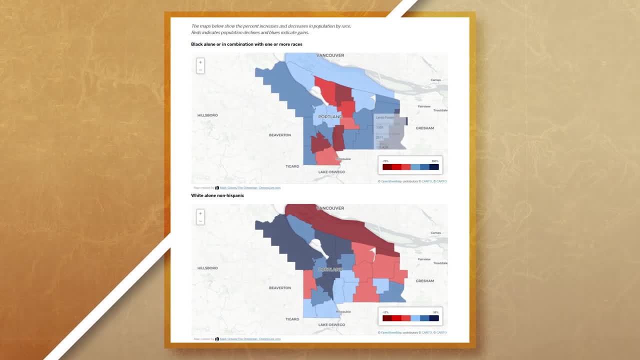 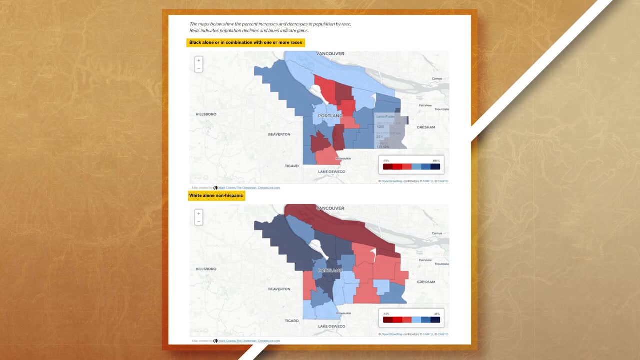 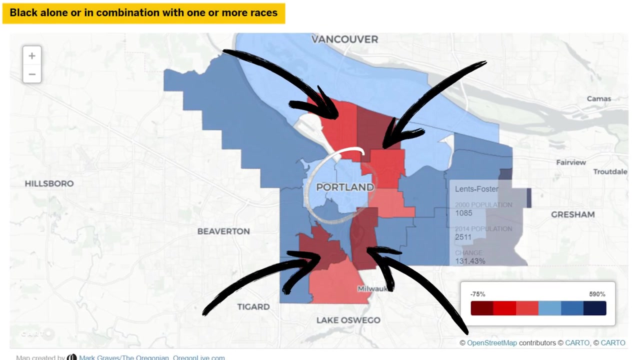 You can see this while looking at this map showing percent increases and decreases by population, by race. The red shows neighborhoods that experienced a decline and the blue shows neighborhoods which gained residents Within just four years. we can see multiple regions near the heart of Portland show a significant decline in black residents with neighborhoods. 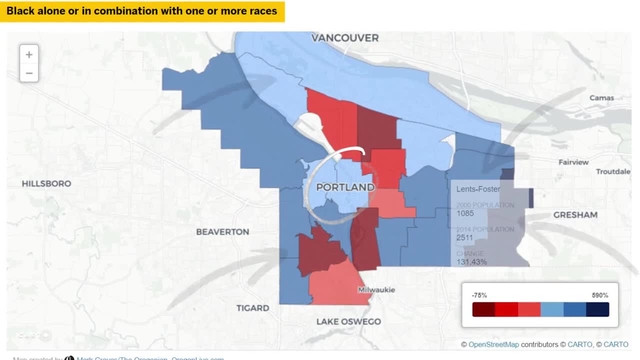 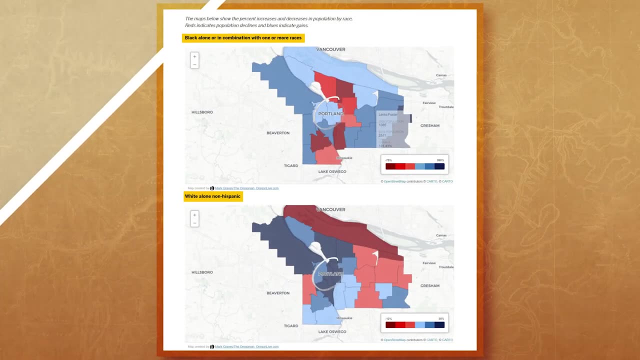 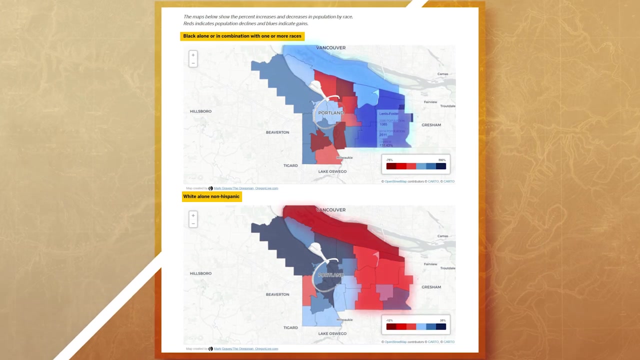 located farther away from the urban core showing the largest increases, While, at the same time, we can see the opposite trend happening with white residents. Notice that the neighborhoods closest to the CBD experienced the highest increases of white residents, while the neighborhoods located farther away from the CBD experienced the largest decreases Today. 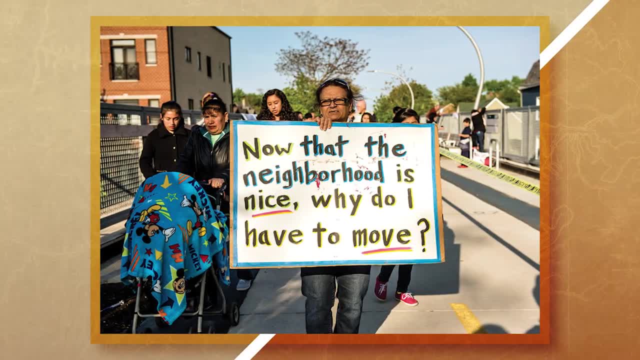 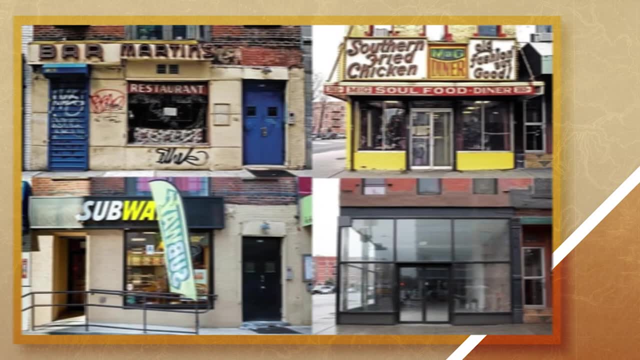 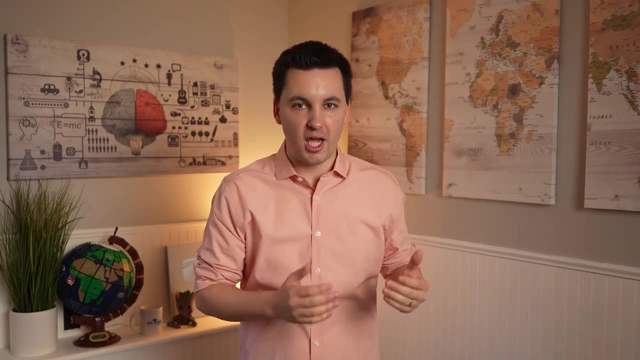 many people also criticize gentrification and smart growth policies for also destroying historical neighborhoods with a unique cultural landscape and sense of place, As new development continues to reshape and replace the spatial layout of cities and their neighborhoods. we will talk more about the causes of gentrification and the impact it has on a 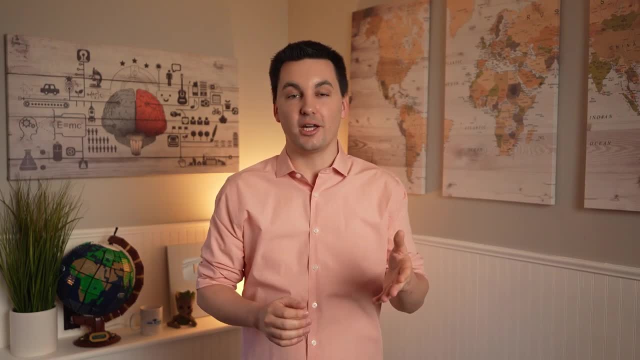 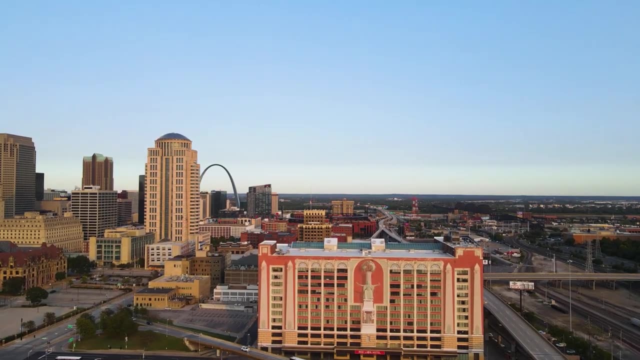 community, and also other impacts, such as redlining, which shifted generational wealth in our Unit 6, Topic 10 video. Another way in which we can see cities, limit sprawl and strive to promote sustainable cities is by adopting policies and practices to limit the pace and scale of new. 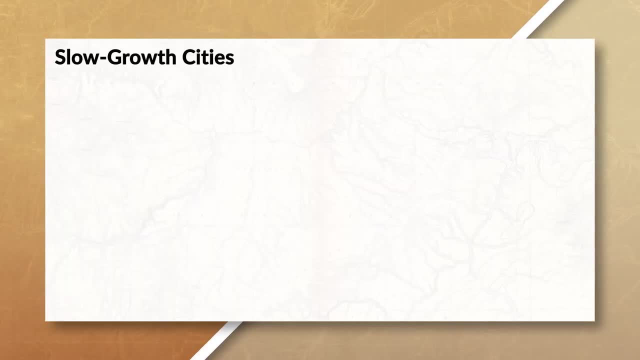 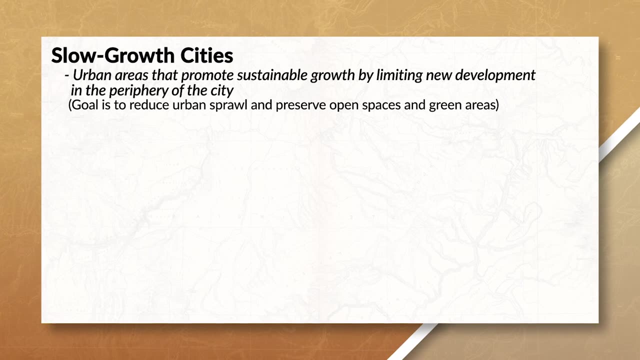 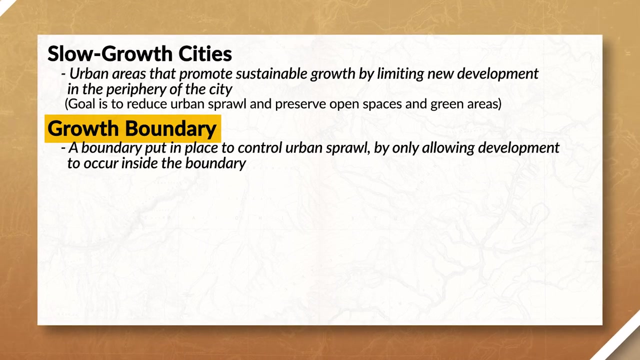 development. These cities are often referred to as slow growth cities. These cities seek to reduce the rate in which their cities grow outward in a variety of different ways. Often times, these cities will implement growth boundaries which restrict the expansion of the city's footprint and prevent urban sprawl, and may even create green belts to protect natural areas. 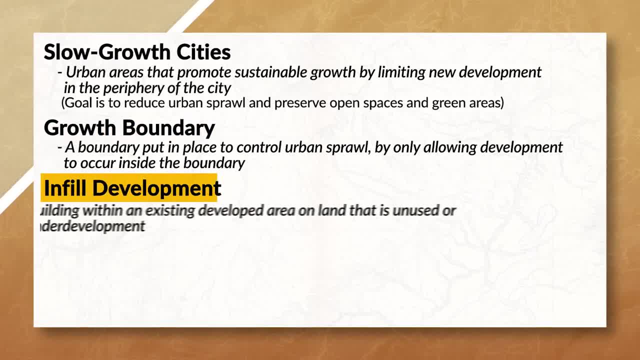 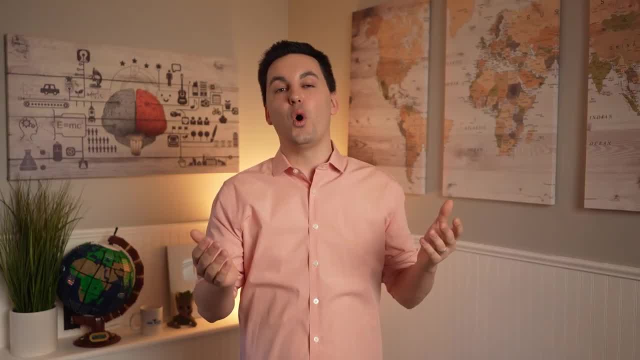 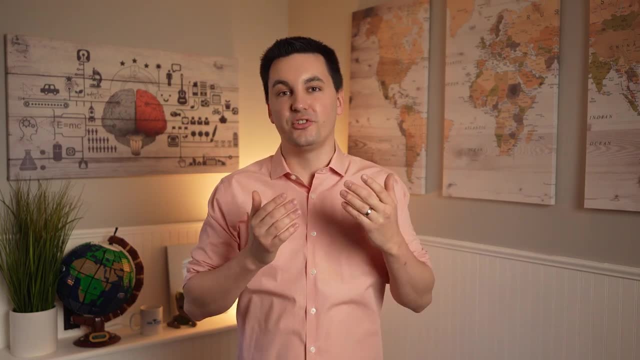 These cities often encourage infill development, which is when cities seek to promote the development of vacant or undeveloped land within an already developed area. This can take the form of developing new buildings on vacant lots, converting older buildings for new uses or redeveloping brownfield sites. This is when cities will implement growth boundaries. 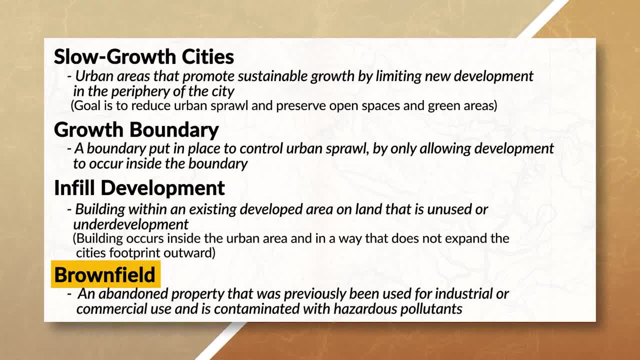 which restrict the expansion of the city's footprint and prevent urban sprawl, and may even create green belts to protect natural areas. This is when land that was contaminated by previously industrial or commercial use is cleaned up and repurposed for new use. We can also see slow growth cities. 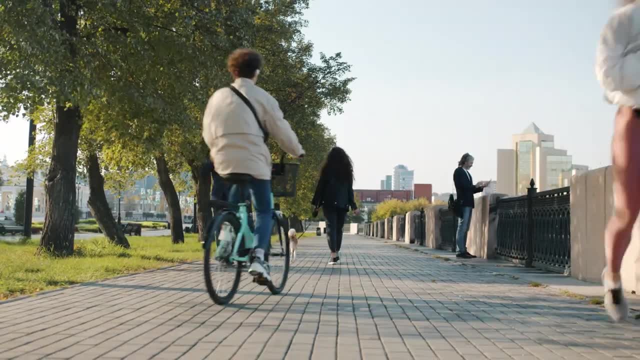 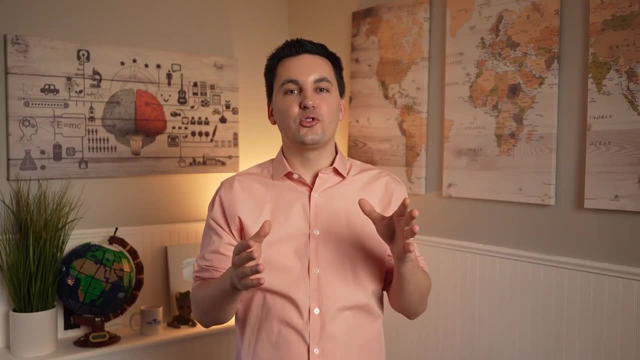 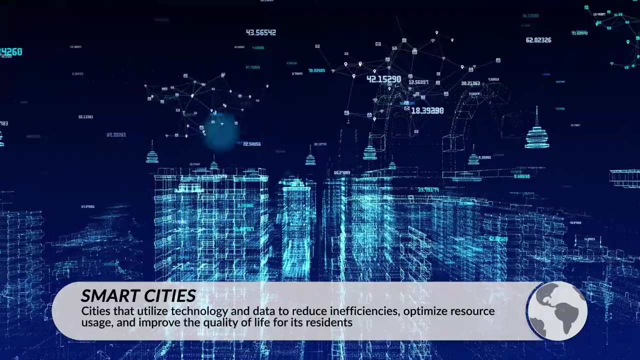 promote public transportation infrastructure for pedestrians and cyclists and other transportation options which reduce residents' reliance on personal vehicles. Today, we are also starting to see a greater focus on creating smart cities, which are cities that utilize technology and data to minimize inefficiencies, optimize the city's resource usage and 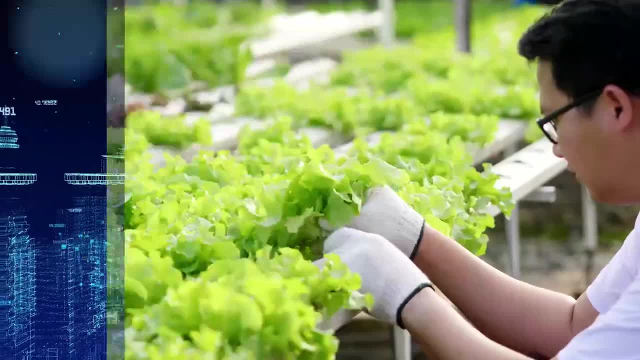 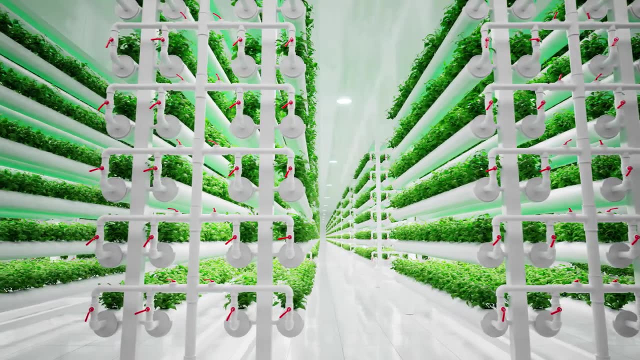 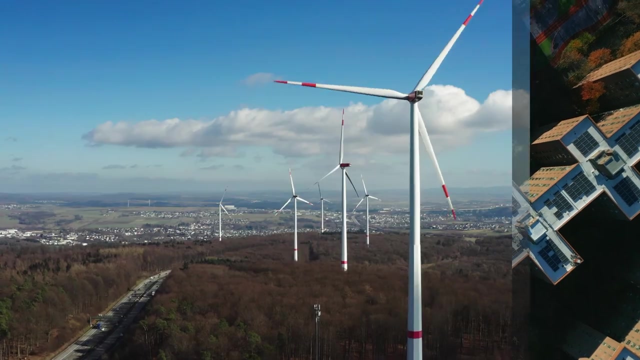 improve the overall quality of life for its citizens. These cities look to reduce the amount of food that is needed to be imported into the city by promoting hydroponics and vertical farming. Smart cities also strive to localize their energy production by utilizing more renewable energy like solar and wind, instead of just relying on oil and gas pipelines.